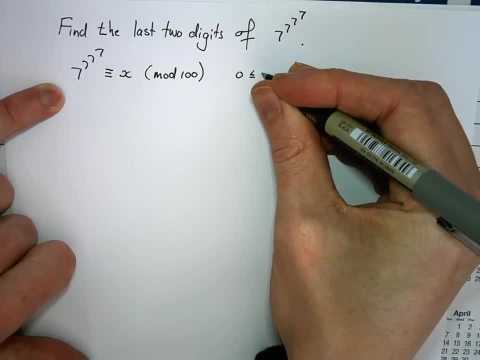 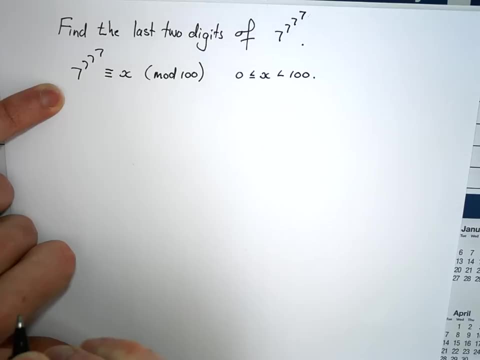 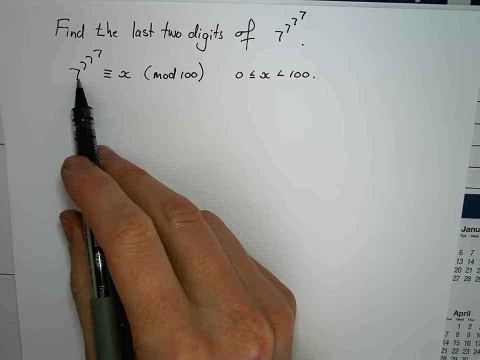 this further and say: okay, this x needs to lie between zero, because 100 could go in exactly, or- and it must be strictly- less than 100.. Okay, now to solve this congruence, I'm going to start looking at the powers of seven And I'm going to see. maybe there's a nice. 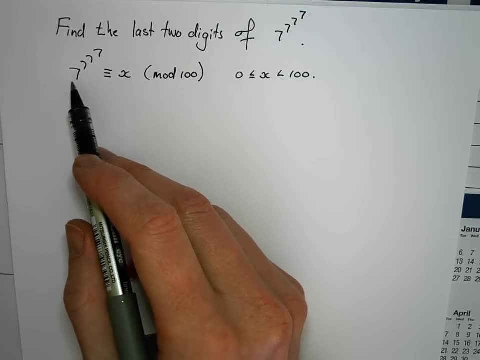 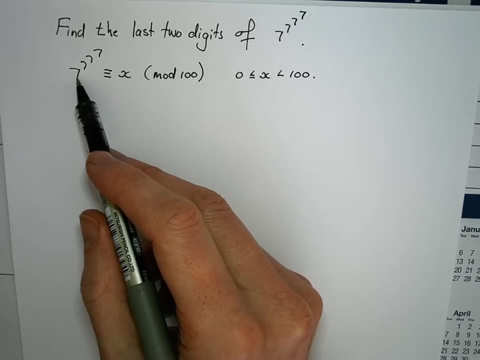 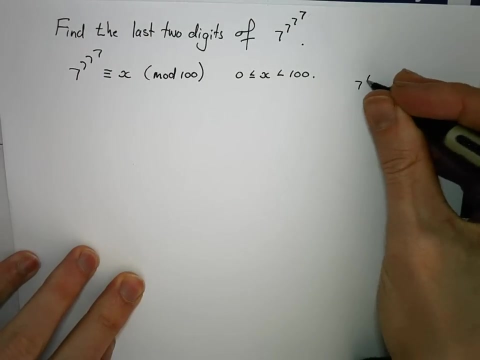 pattern if I look at the successive powers of seven modulo 100. Or maybe I can find a power of seven that is particularly easy to work with modulo 100. So I start looking at these things. I say, okay, seven to the power one. Well, that's just congruent to seven modulo 100. It doesn't. 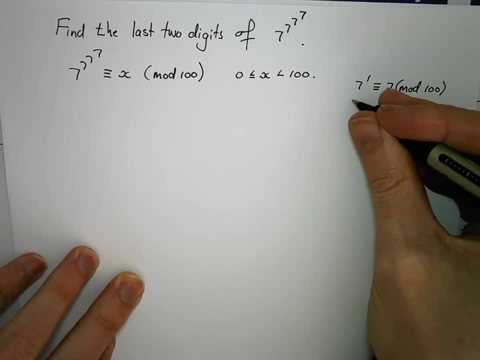 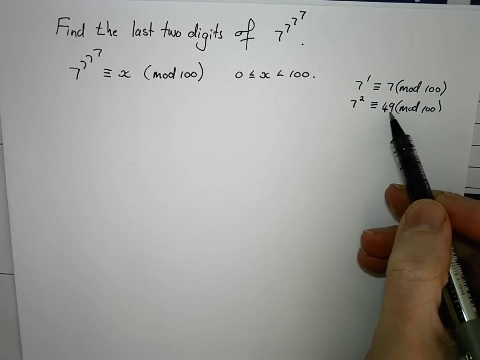 really reduce to anything easier. Seven to the power two, Well, that's 49.. That's just congruent to 49, modulo 100.. I could add and subtract multiples of 100 to 49.. Of course that would give me other things congruent to this modulo 100. But you can try and you can see it's not. 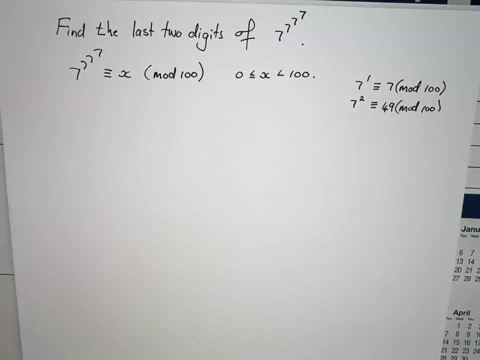 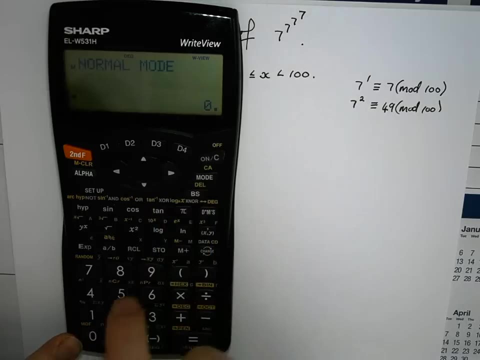 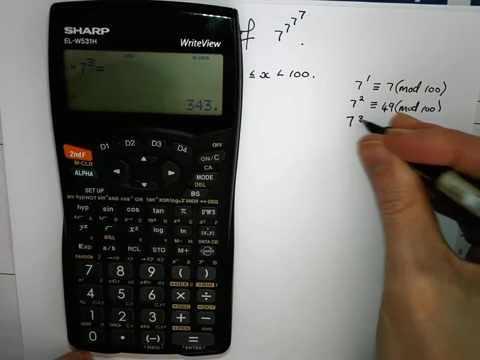 really going to work very well. Now, seven to the power three. Let's check that. If you don't remember that, you can use your calculator. Seven to the power three, it's going to go as 343.. Seven to the power three, three, four. well, it's equal to 343,. 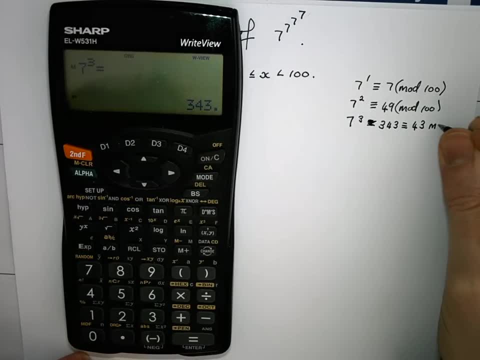 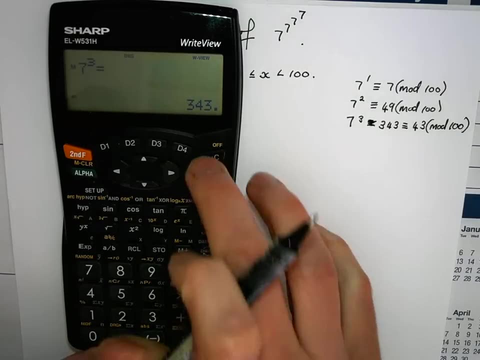 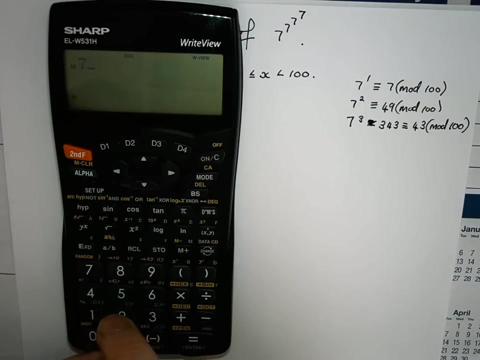 which is congruent to 43, modulo 100.. Okay, well, 43,, 49, seven. nothing is really looking very promising. So at the moment we can't really see a pattern emerging yet. Let's try. seven to the. 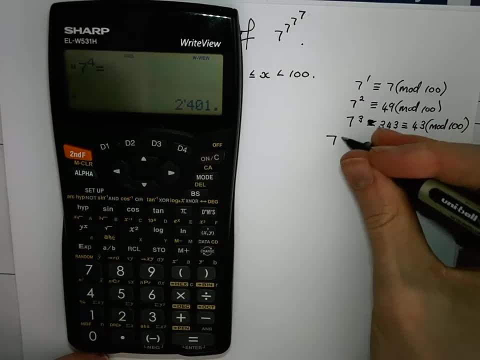 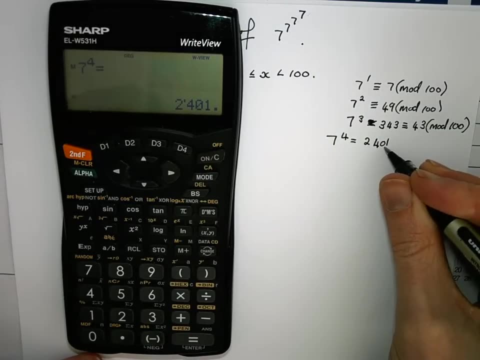 power four. So seven to the power four is equal to 2401.. And now we strike the jackpot, because modulo 100, this thing is just congruent to zero. If I divide by 100, the remainder is zero. So this thing is congruent to one modulo 100. And any power of one is, of course, 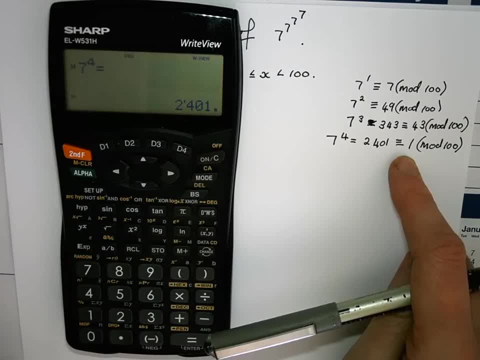 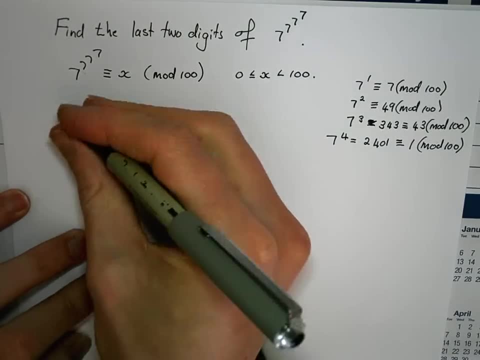 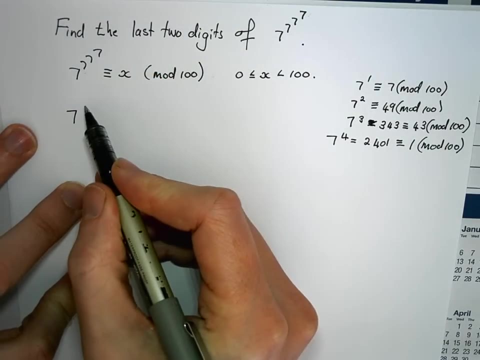 extremely easy to work out. It's just one again. So I want to exploit this fact to try and solve this congruence over here. So what I want to do is I want to say: well, suppose I could write this seven to the seven to the seven, as something times four plus the remainder. I can do that. 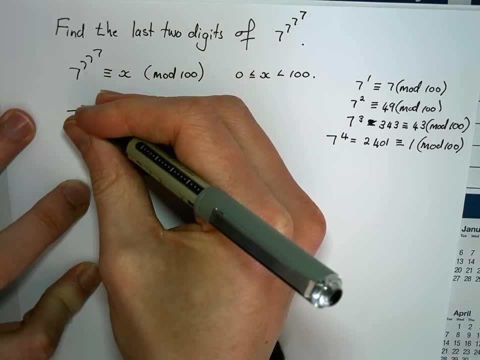 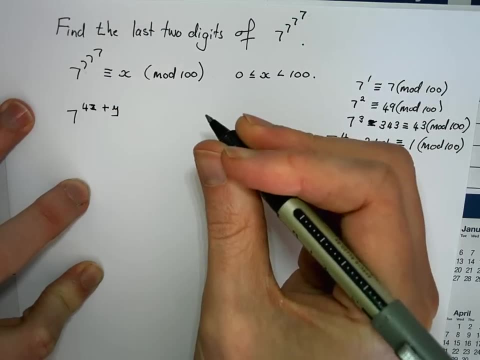 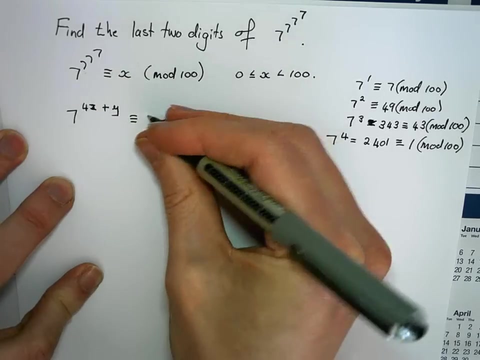 with any number. So suppose four goes in x times. Let's say it goes in z times and leaves the remainder of y. Okay, If I could do this this well, I've just rewritten that that would be congruent to x modulo 100. 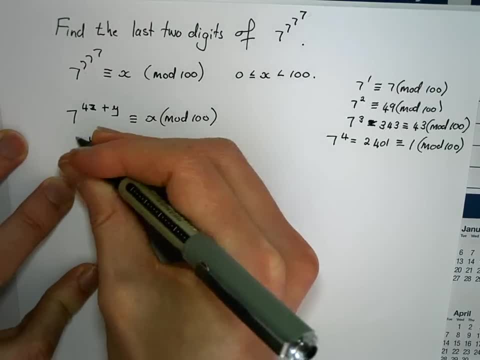 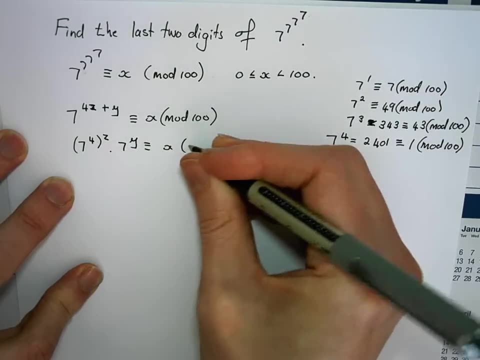 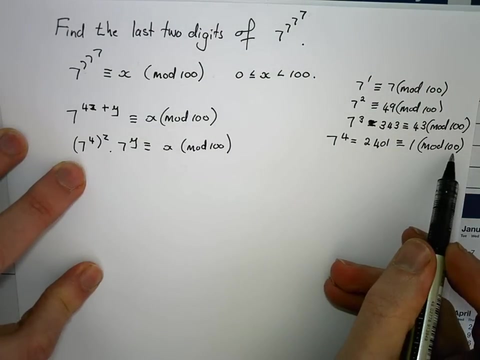 Then I could say: look, this is seven to the four, all to the z, times seven to the y. I've just used my laws of exponents over there. And now this: well, this thing is congruent to one modulo 100.. Properties of congruences, tell us. 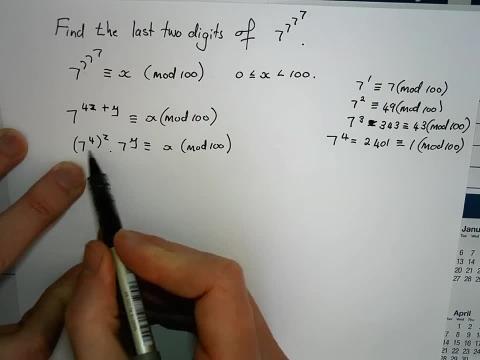 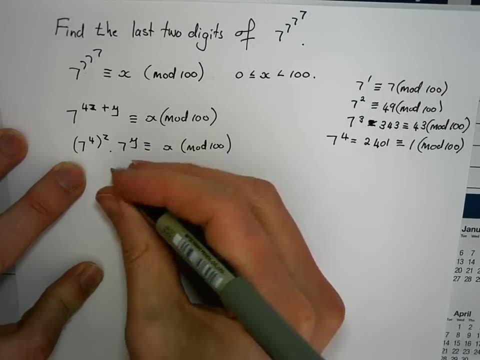 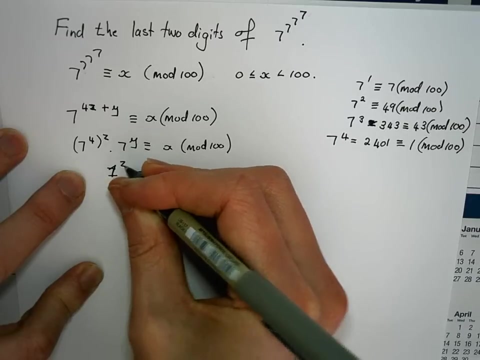 that in I can replace in powers, congruence with congruence, And in products, I can replace congruence with congruence, And what I'll get will be congruence. So this will give me seven. This will this, in fact, will give me one to the power z times seven to the power y. 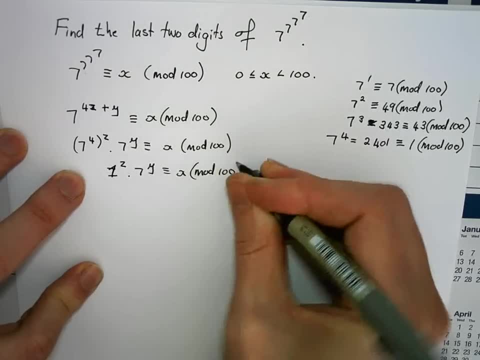 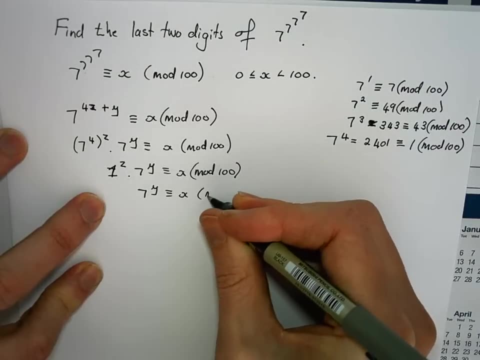 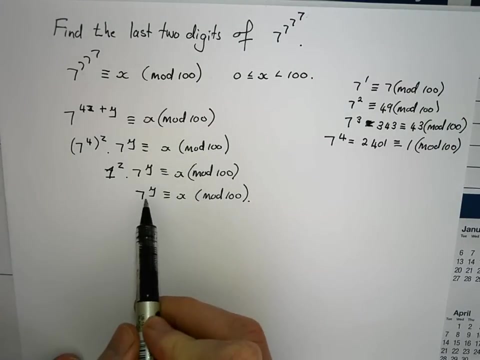 And that will stay congruent to x Modulo 100.. And one to any power is just one, So this will reduce to seven, to the y, Which would be congruent to x modulo 100.. All right, So then this is. this is looking much. 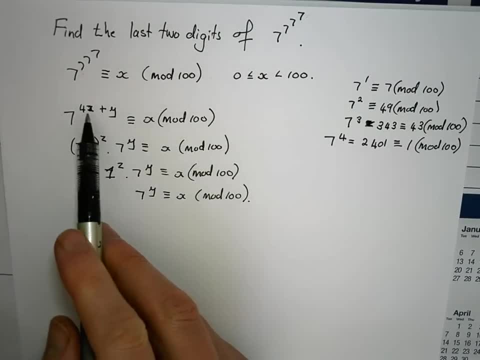 much better. Okay, Because particularly y here, whatever I've done here, I've divided this exponential tau of seven to the seven to the seven by four, And I expressed it like this: Four went in z times And left a remainder of y, So y over here is going to be something between zero and three. 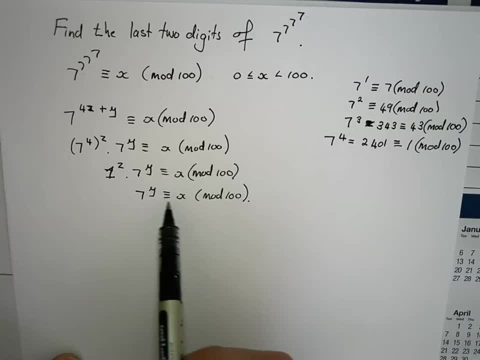 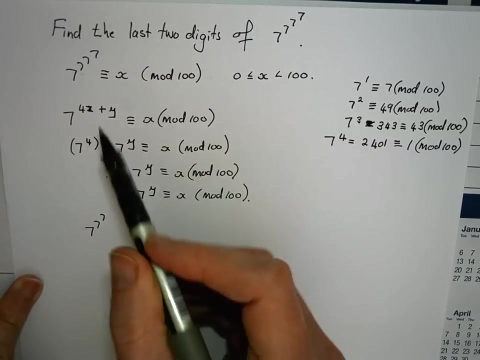 So that's very easy. If I can find this y, this congruence is going to be very easy to solve, Much easier than the one we started out with. So what I need to do is I need to find this y. So what have I done here? I wanted here seven to the seven to the seven. Notice I'm only taking. 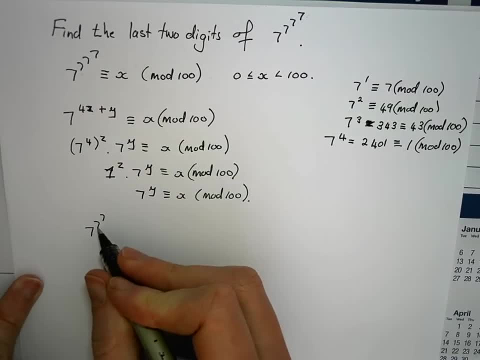 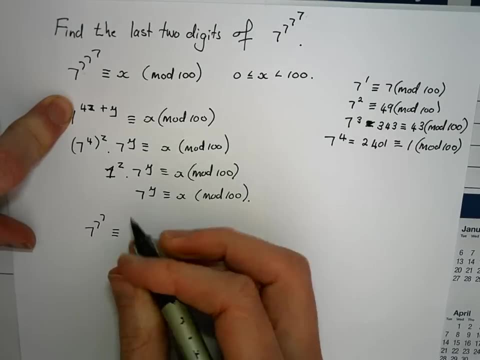 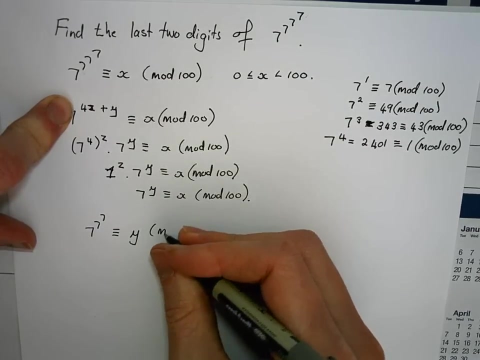 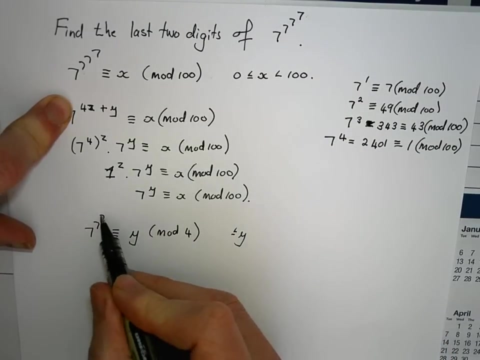 the exponent here. I wanted to write this thing As something times four plus y. So what I'm looking for is: I'm looking for the remainder if I divide this thing by four. So I'm looking to solve this congruence And, of course, again, where y is the number congruent to this thing, modulo four, which is: 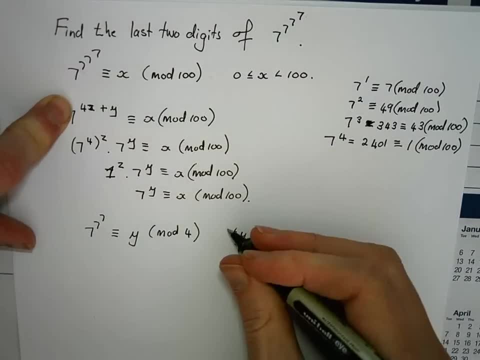 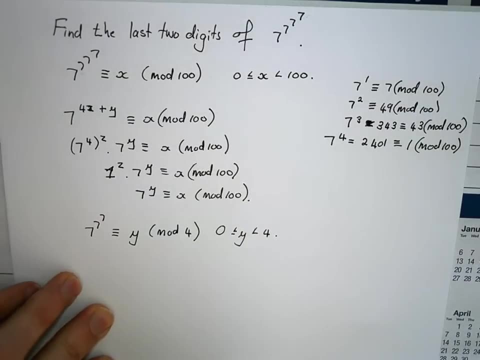 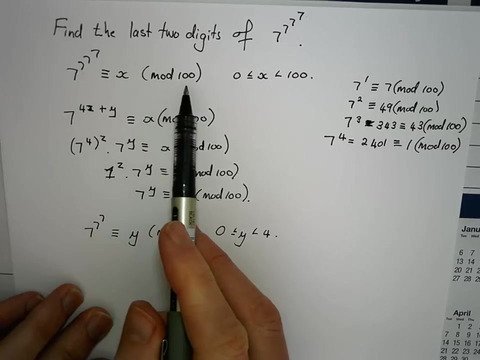 the remainder of the division of this number by four. So particularly it needs to lie between the bounds Zero and strictly less than four. All right, So notice, here we're apparently changing base. here I was working modulo hundred here, And now I'm working modulo four. The point of working modulo hundred here is that 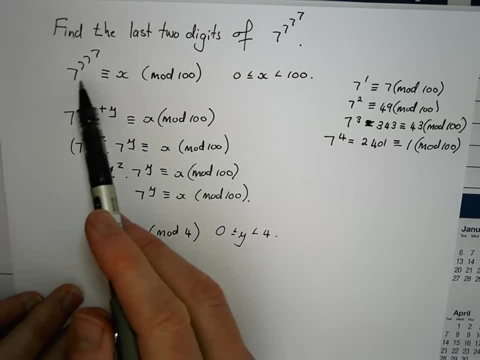 I want the last two digits of this thing, So the remainder of this thing after division by a hundred, To do that. I noticed that, well, if I could rewrite the exponent part of this, I would be able to do that. So I'm going to do that. So I'm going to do that. 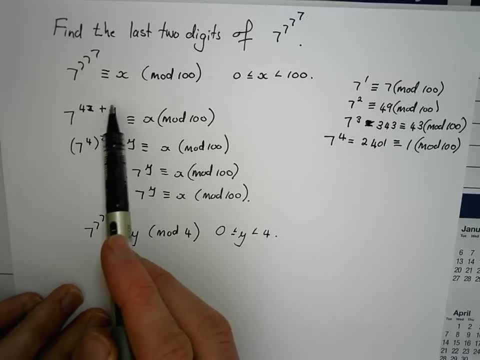 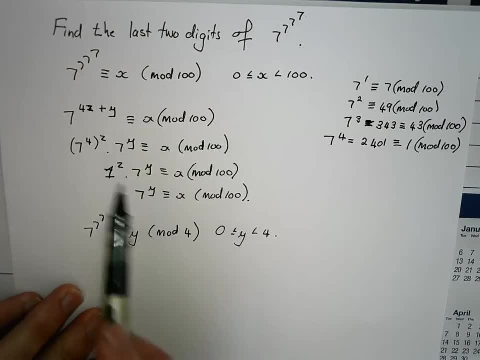 ating b I B. So for instance, if I wrote the past James Bond line, I would get this as something times four plus y. The y is the remainder of the division by four. then this would all reduce to that. 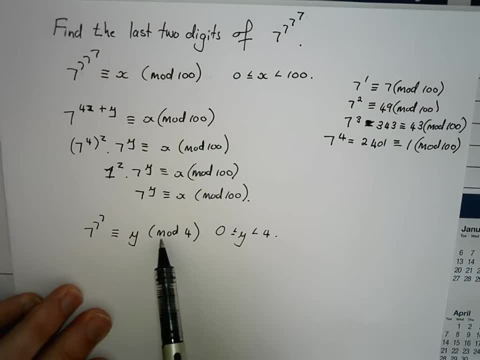 So now I'm working to try and find that y which I can then plug back in there. So this: I'm finding a remainder of the division by four. again going to start, I'm going to look at powers of 7, modulo 4, and see if I see a pattern, or 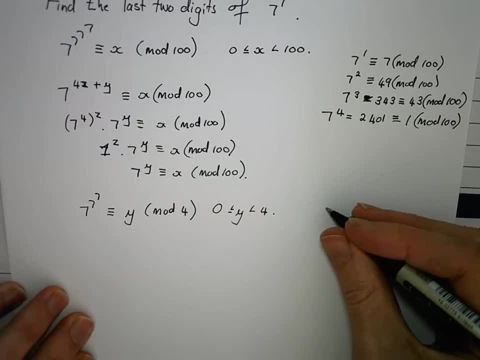 something that works particularly easily, All right. so I'm going to say 7 to the power 1,. well, that's just congruent to 1.. Just congruent to 7.. Mod 4,: it's also congruent to 3 mod 4,. 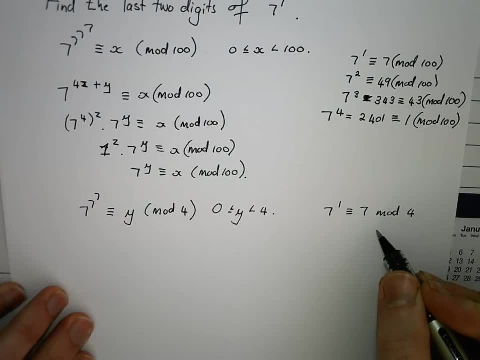 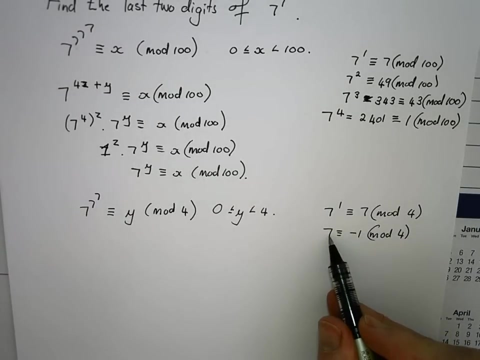 it's also congruent to minus 1 mod 4.. Okay so yes, look at this: 7 is congruent to minus 1 mod 4, right, Because if I take 7, I can subtract 4, it gives me 3, so something congruent mod 4.. 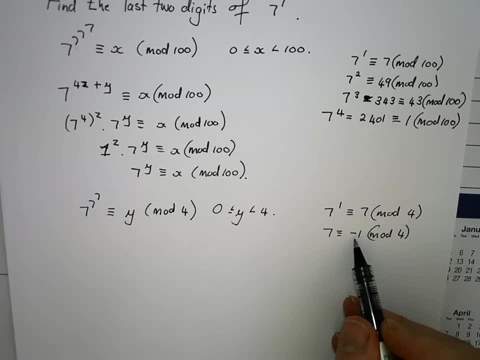 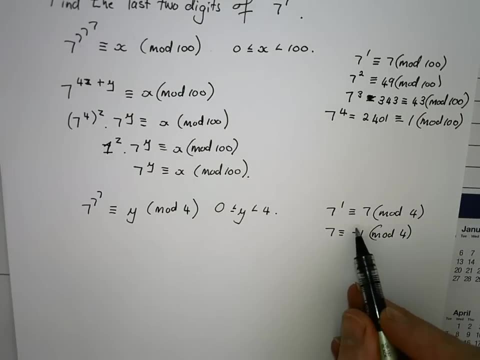 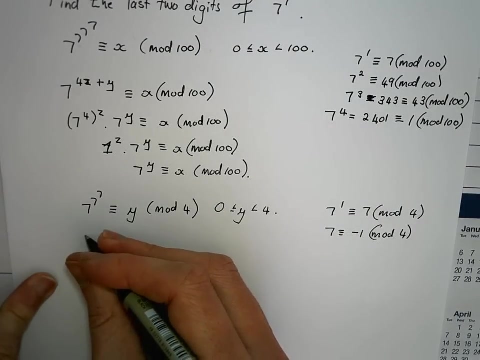 From 3, I can subtract another 1,, another 4, which gives me something congruent: mod 4, minus 1.. Now, any power of minus 1 is very easy to work with. so this guy is, in fact, this is, minus 1. 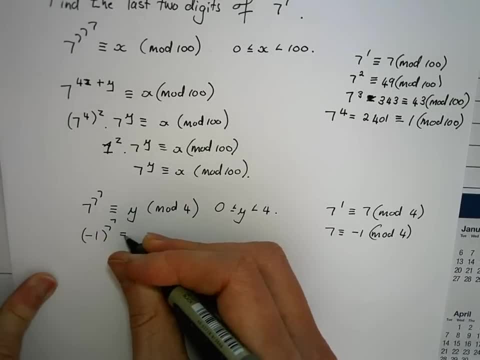 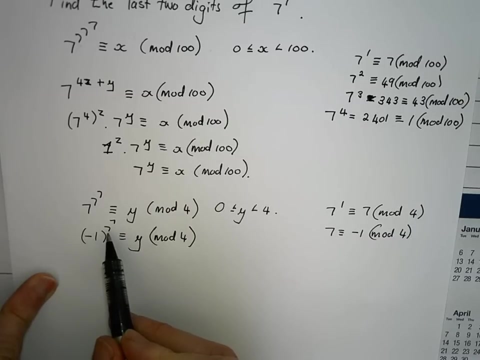 to the 7 to the 7, would be congruent to y mod 4.. All right, now, what is this? This is an odd power, because I've got 7 multiplied with itself 7 times. This is going to be an odd number. 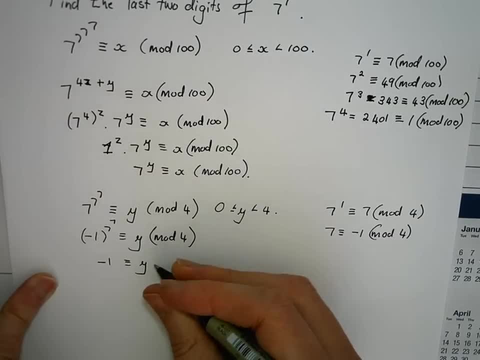 so this is going to give me minus 1 mod 4.. Okay now, of course, this is not. this doesn't satisfy this, so I need to work back to something within that range which is congruent mod 4.. I can add 4 here, which is going to give me: 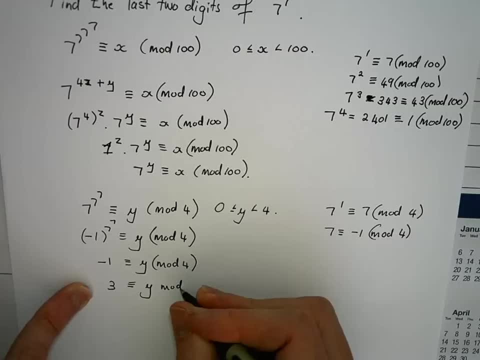 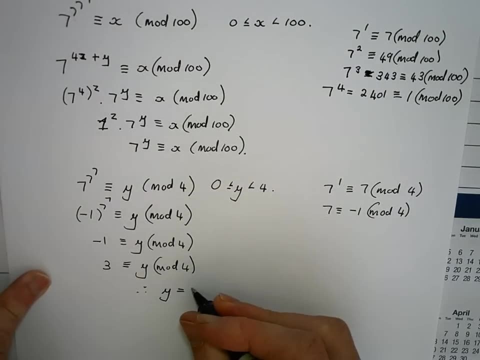 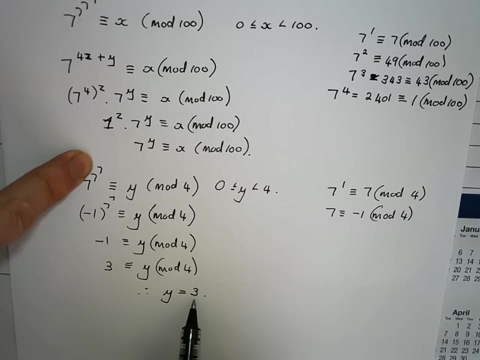 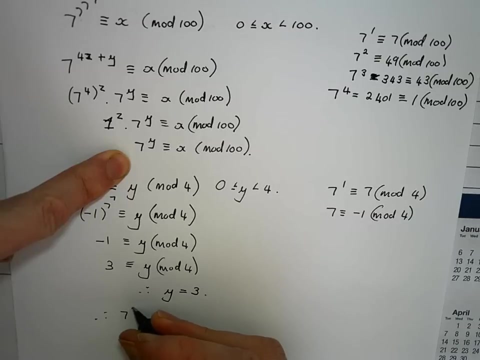 3. Okay, so particularly I can take y to be equal to 3.. Okay, this means if I divide this exponent by 4, the remainder is going to be 3.. So I can take it back here and say: well, this means 7 to the 3 is congruent to x modulo 100. 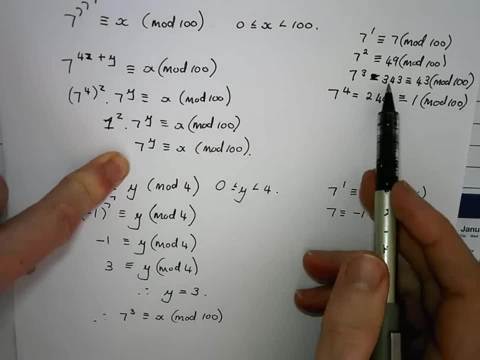 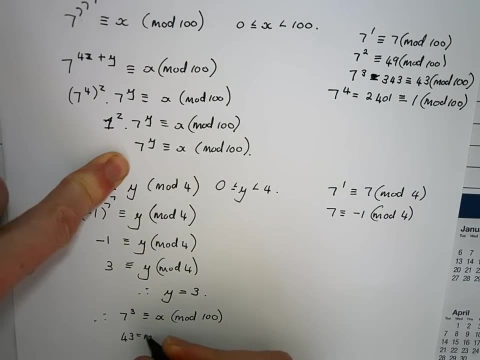 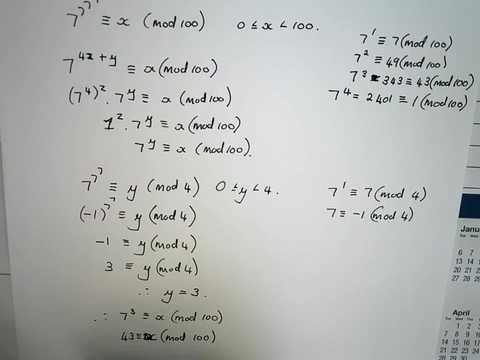 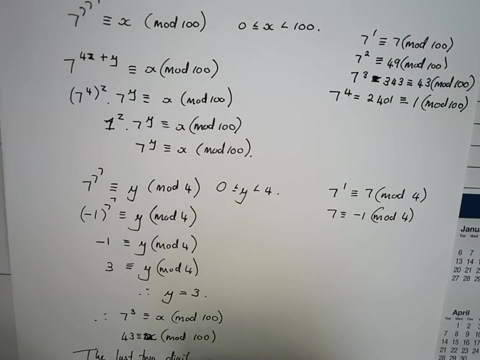 We've already looked at 7 to the 3.. 7 to the 3 is just 43.. 43 is congruent to x modulo 100, and 43 falls within the bounds that we're interested in. So we conclude that the last two digits of 7 to the 7 to the 7 to the 7 are: